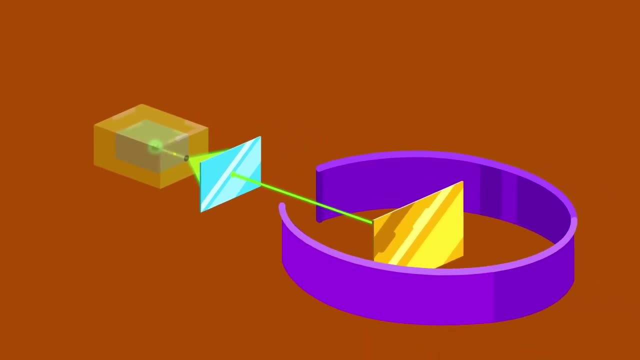 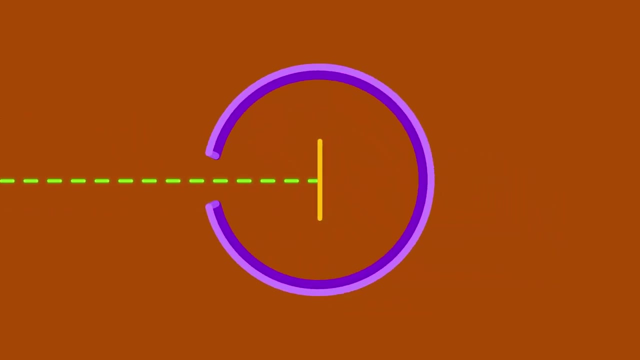 charged alpha particles through it. The box was positioned in line with the thin gold foil that was surrounded by a zinc sulfide screen. While the alpha particles from the radium hit the gold foil, they scattered and produced light flashes that were detected by the 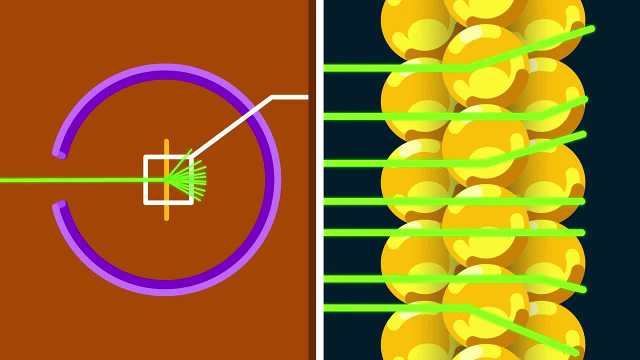 screen Based on the plum pudding model. Rutherford thought that most of the particles would pass through the foil, while some are slightly deflected due to their encounter with electrons. Initially, the experiment results were indeed consistent with his assumption, But what followed next was totally unexpected. Some particles encountered large-angle deflections. 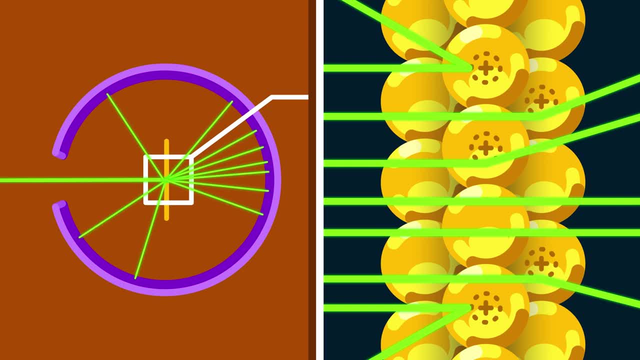 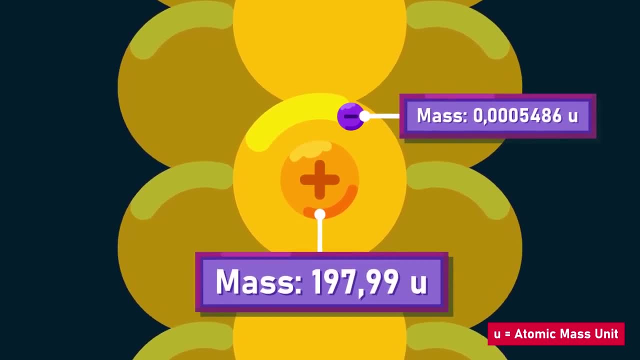 and very few, about one in every 20,000, were bounced backward. Rutherford thought there must be something positive, minuscule yet heavy in the center of gold's atoms that repels positive alpha particles and essentially makes up the atomic mass. 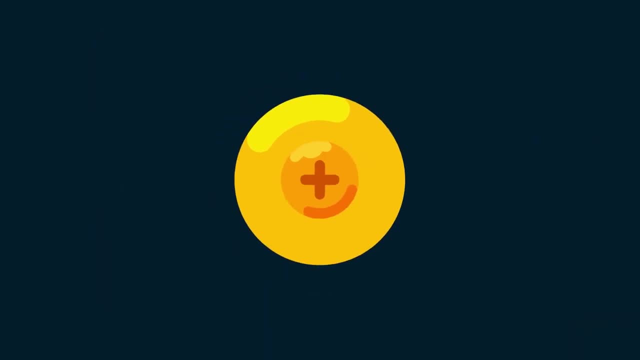 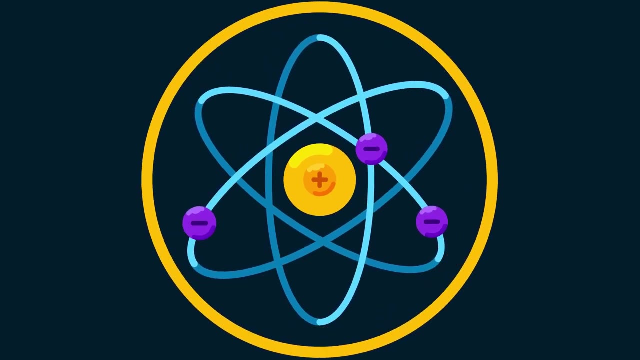 He called it the atom's nucleus. The results strengthened the previous notion about the existence of positively charged particles, later known as protons, within atoms, And, since the majority of the particles pass through, he suggested that an atom is mostly empty space. 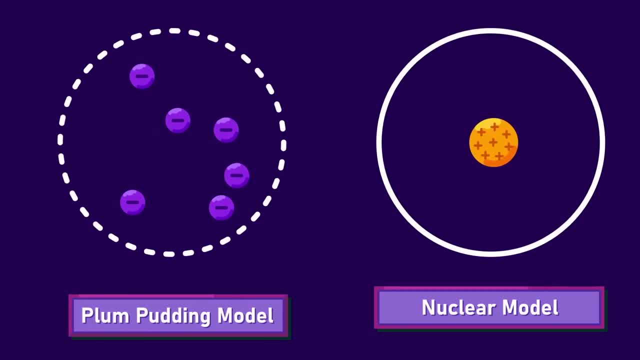 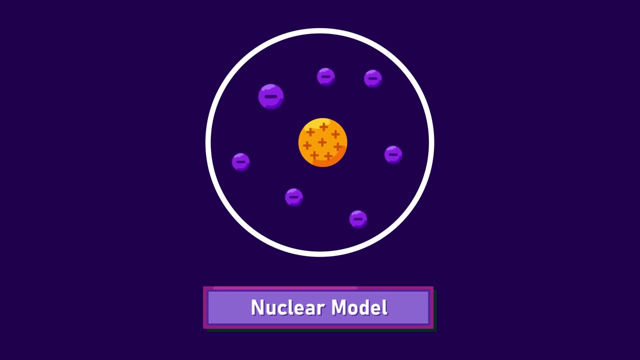 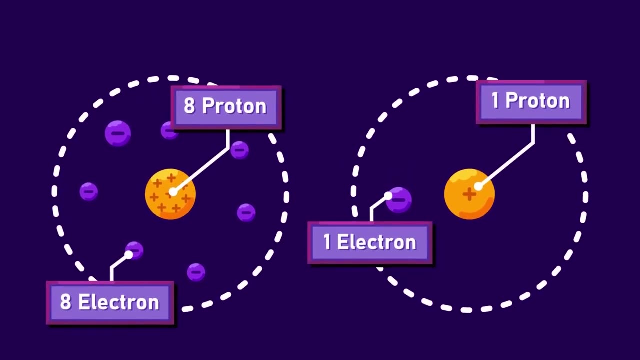 Rutherford proposed an atomic model named the nuclear model, based on this inquiry. He stated that this is a tiny nucleus with positively charged particles inside and it is surrounded by electrons. Different elements have different numbers of protons, but in one atom the proton amount is equal to the number of electrons revolving around the nucleus. 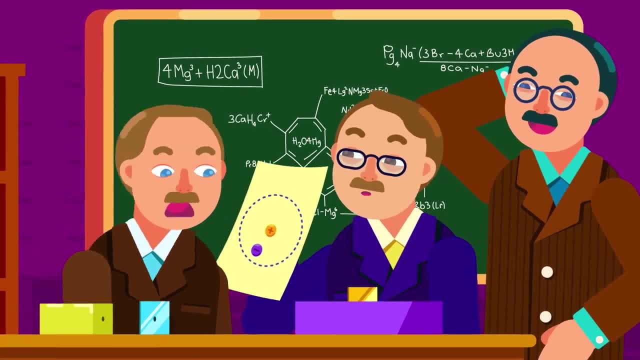 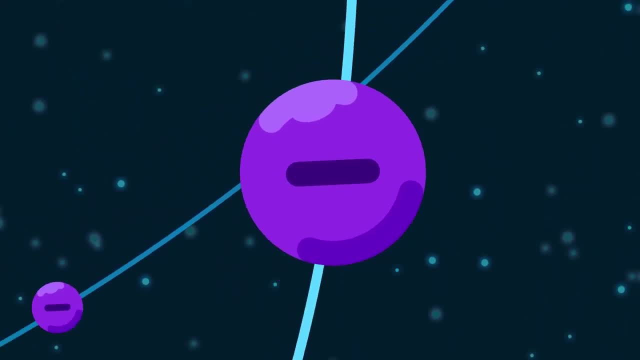 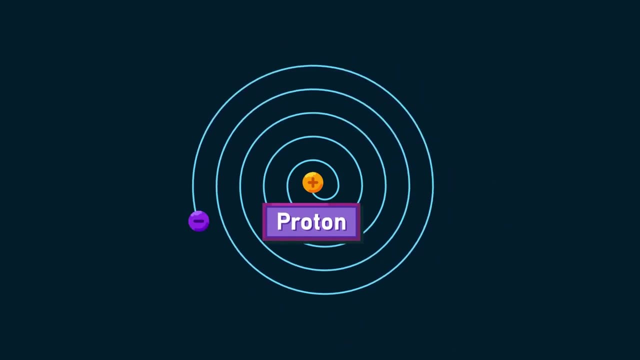 making the atom neutral. This model satisfyingly answered the questions that plum pudding model couldn't explain, But it contradicts the principle of classical electrodynamics. According to the principle, a charged particle in circular motion radiates energy continuously. The electrons in this model move in circular motion and lose energy. 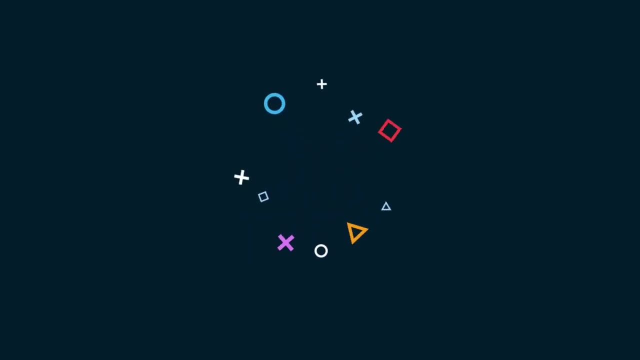 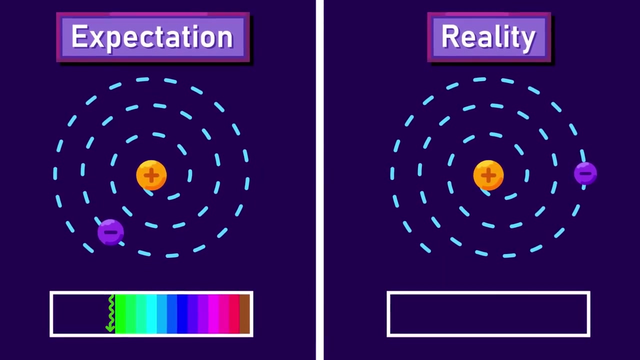 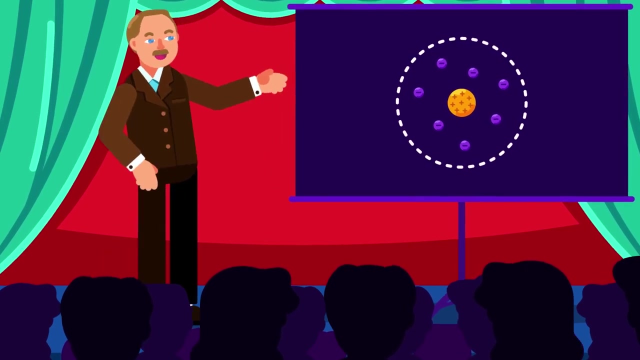 Causing them to spiral toward the center and resulting in the collapse of the atom. Yet in fact, none of these things happen. Additionally, the energy radiating particle must form a continuous atomic spectrum, But the observation showed a line spectrum. Despite the limitations, Rutherford's model provided a fundamental understanding of atomic 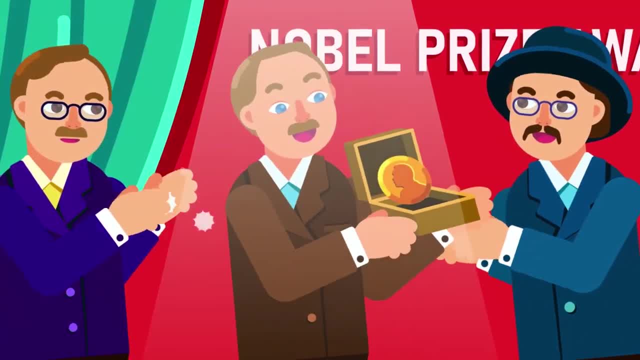 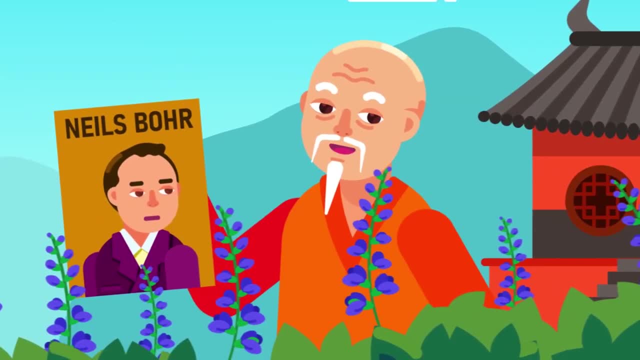 structure. His intensive research about atoms and initial discovery awarded him the Nobel Prize. We are still halfway through our journey on atomic model development. In the upcoming video, as you guess, we'll move forward a few years later to discuss the next model and how.